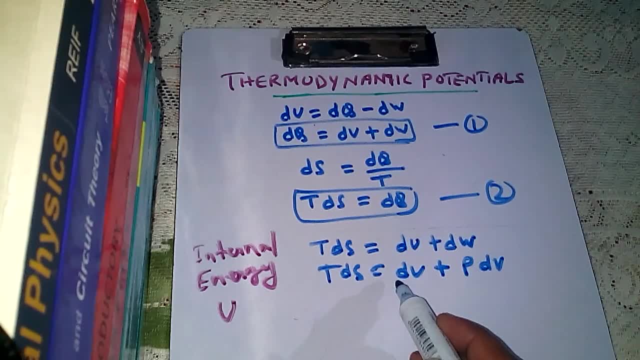 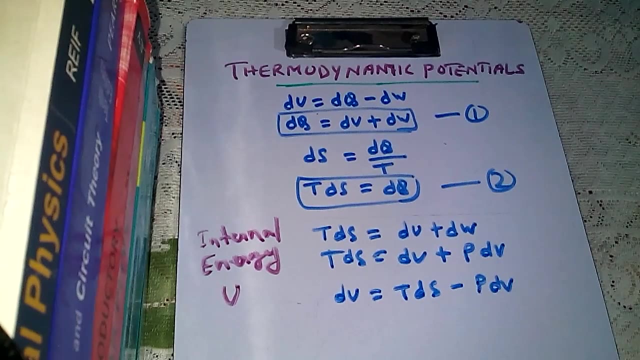 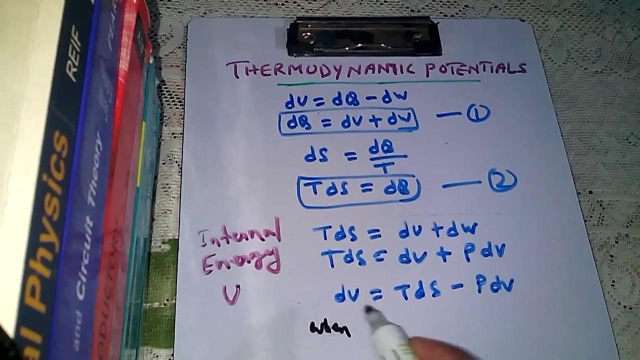 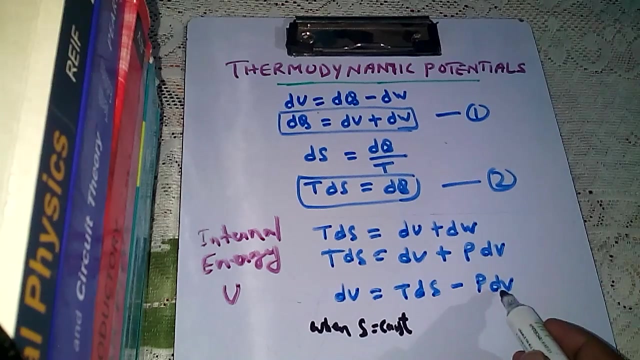 Since we want to find u. so let us take this term du to the left hand side, So du is equals to Tds minus Pdv. Now from here we can have two relations When we take entropy as constant And volume is variable. 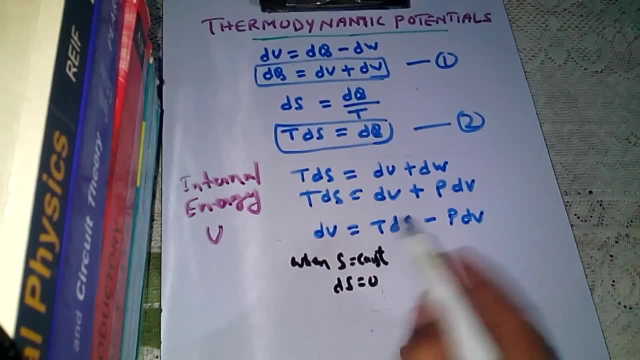 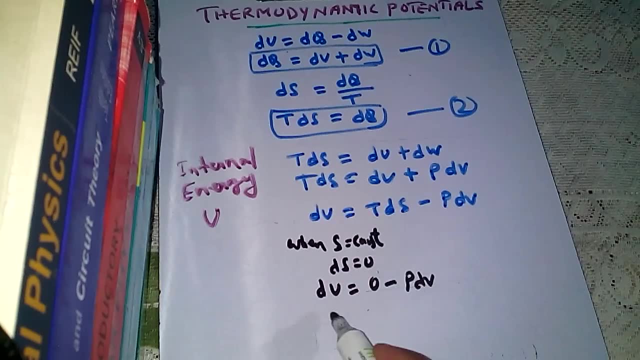 Then ds is equals to 0. And under this condition this relation becomes du. equals to this part is 0 minus. this is Pdv. So from here we have: P is equals to minus of del u by del v, And this is possible under constant. 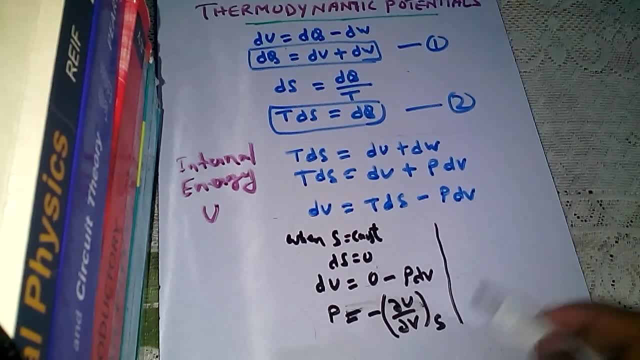 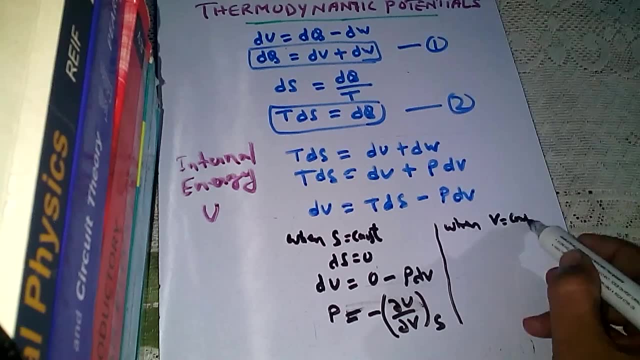 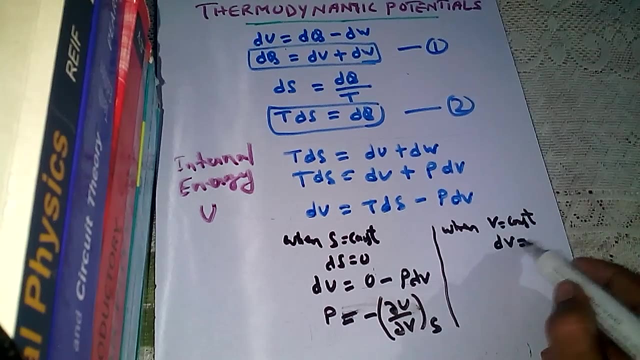 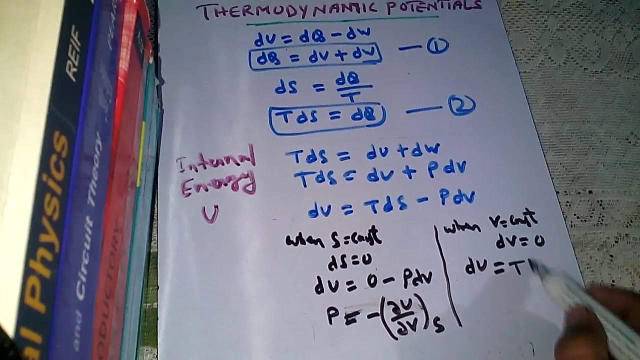 Now we can have the second relation, when we take: volume is constant, but entropy is variable. So under this case dv is equals to 0. And then this relation becomes: du equals to Tds and this part is 0. And now we have: 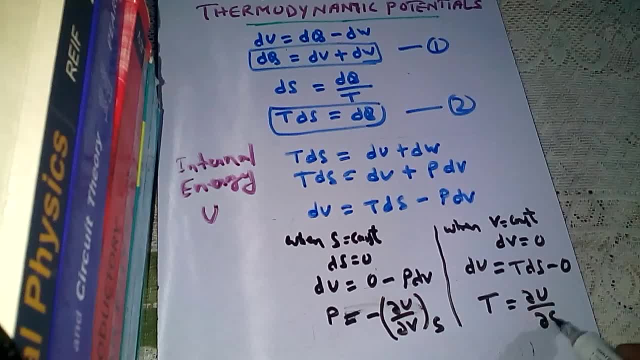 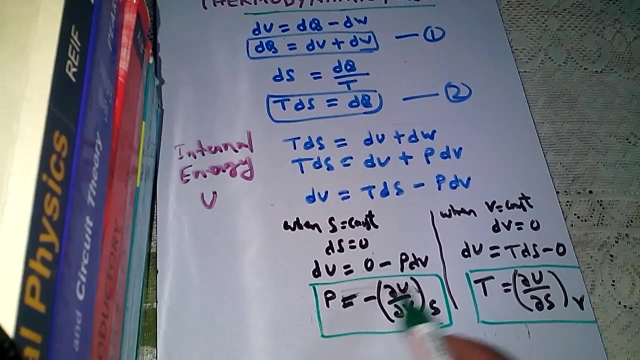 Tds is equals to del u by del s under constant volume. So we have two relations, And you should remember this, relations. So this says that pressure is the rate of change of internal energy with respect to volume under constant interval And it says the temperature can be given as the rate of change of internal energy with respect to entropy under constant volume. 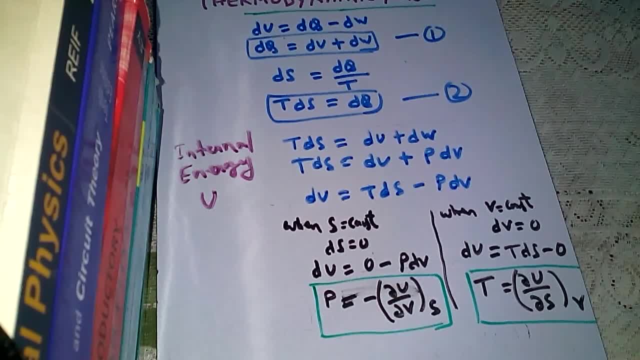 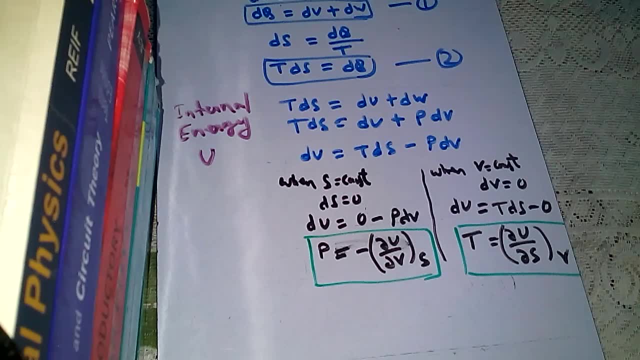 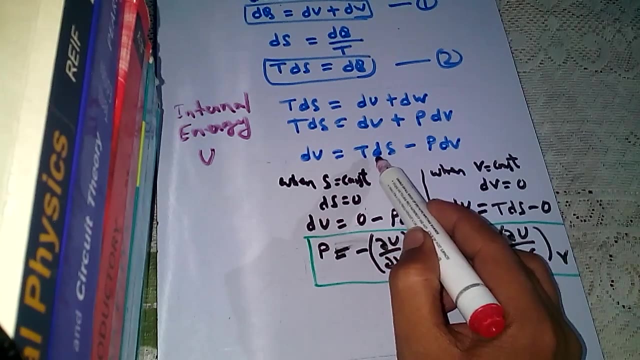 Now let us move to our next potential, That is enthalpy. Now one more thing to be noticed: that, since from here we see, du is equals to Tds minus Pdv. And here, what are the variable terms? Only entropy and volume. 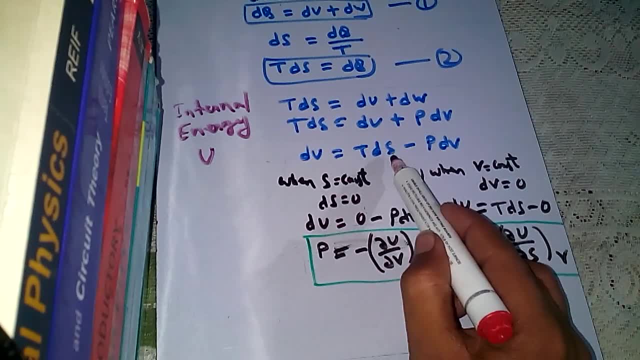 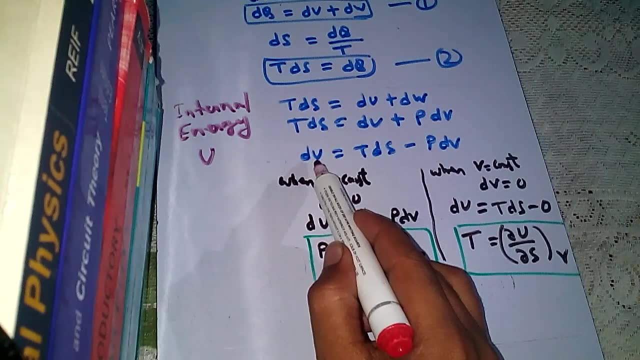 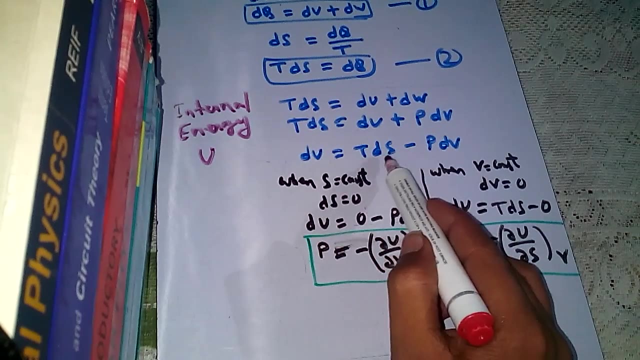 Because Temperature and pressure are constant now. So entropy can change and volume can change. And this is the final relation for the internal energy. I should just change in internal energy. Okay, So this change in internal energy actually depends on the change, on change of entropy and change of volume. 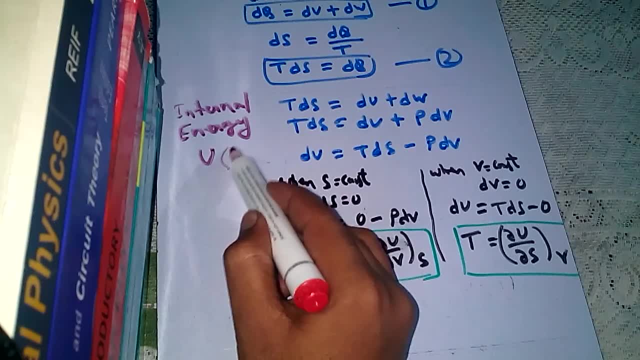 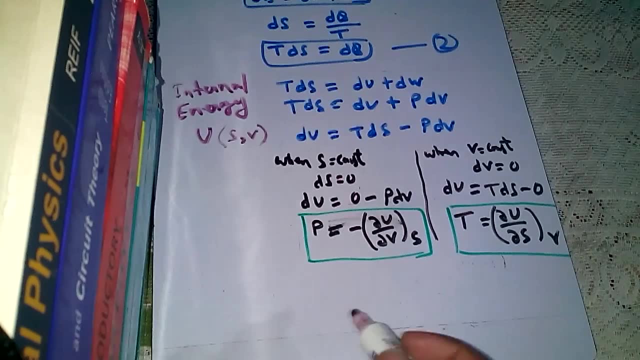 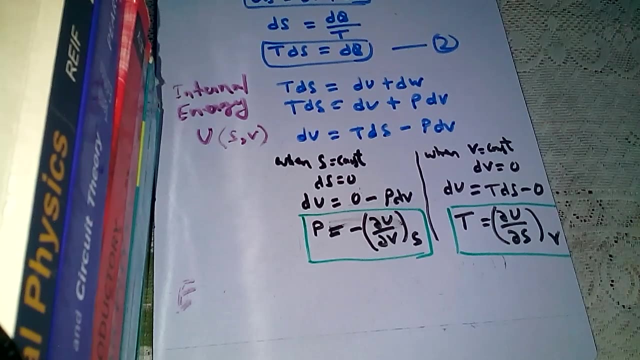 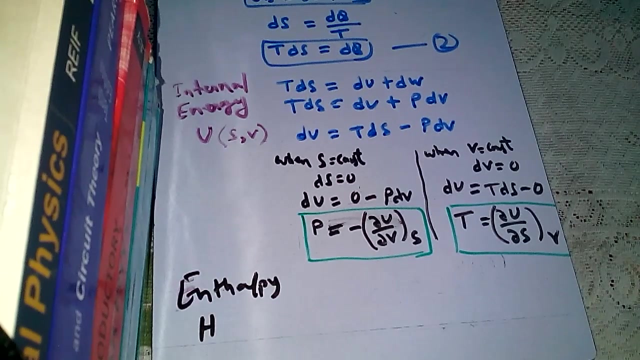 And that is why we say that internal energy is a function of entropy and volume. Okay, Now let us go to our next potential, That is enthalpy, And this is given by H, Capital H, And we already know the formula for enthalpy. 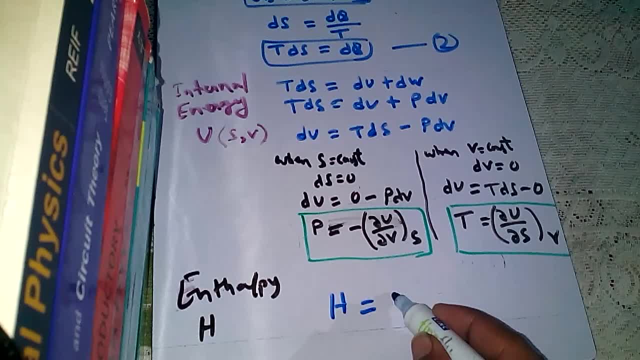 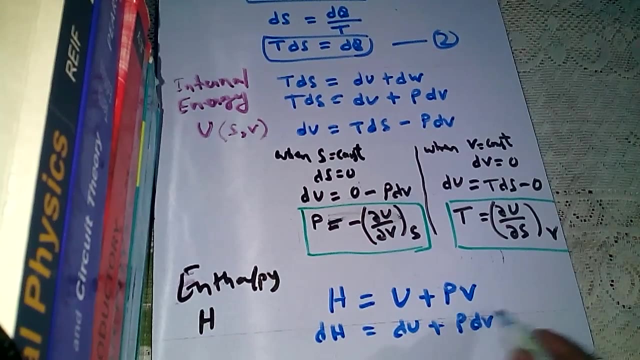 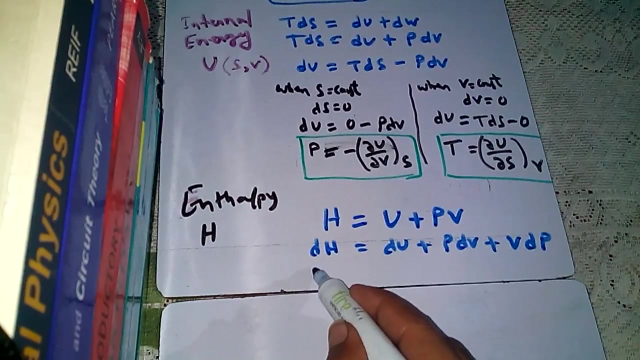 H is given by U plus P into V. Now what we will do. We will differentiate on both sides, So it will become: dH is equals to du plus Pdv plus Vdp, So we will have: dH is equals to: 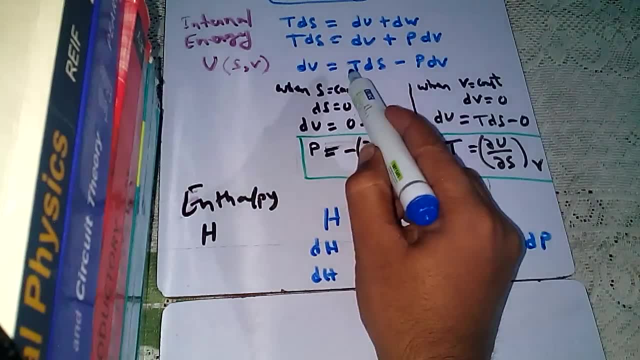 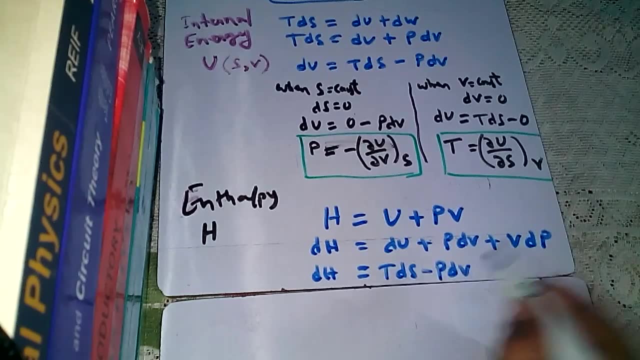 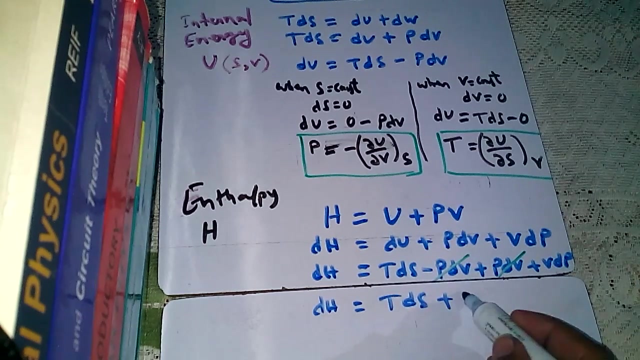 Now du, we will put from here. So it is Tds minus Pdv, Then plus plus Pdv, Pdv plus plus Vdp And we can see that minus Pdv plus Pdv cancel each other. So we have dH is equals to Tds plus Vdp. 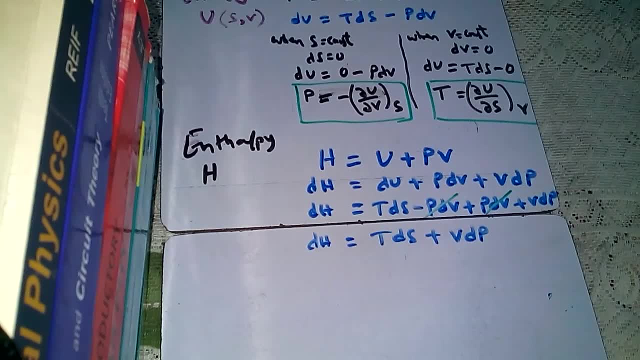 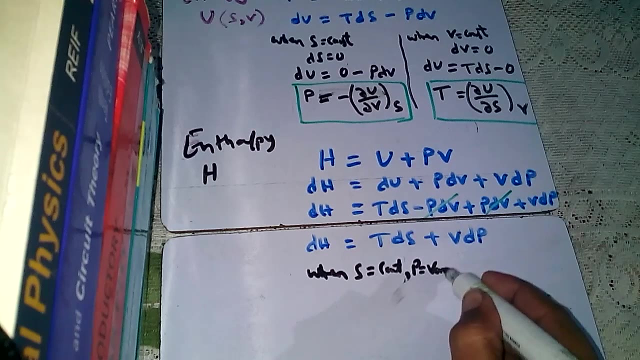 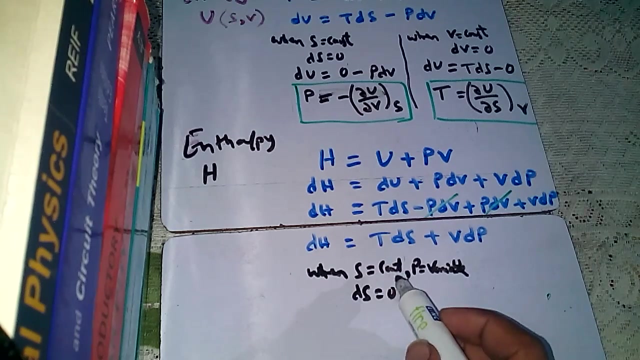 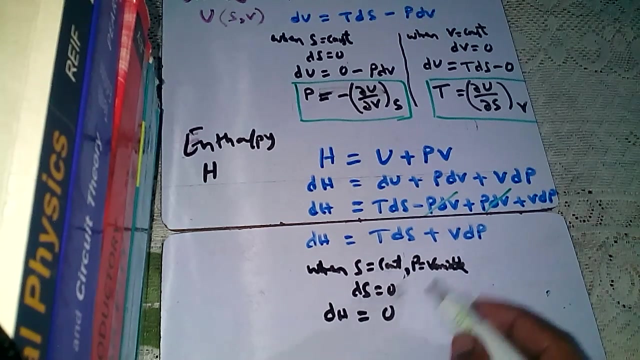 Now again we can have two relations. So the first condition: when entropy is constant and pressure is variable, We can write: pressure is variable And under this condition dS is equals to 0. So this relation becomes dH equal to 0 plus Vdp. 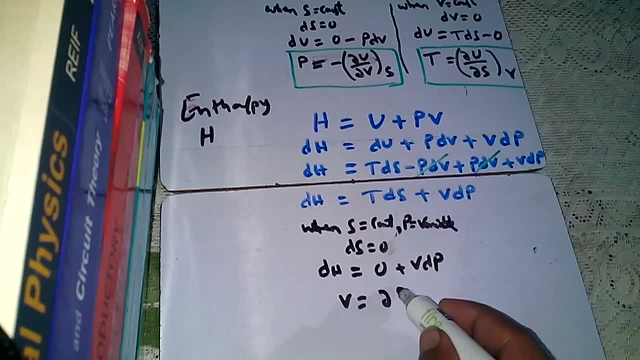 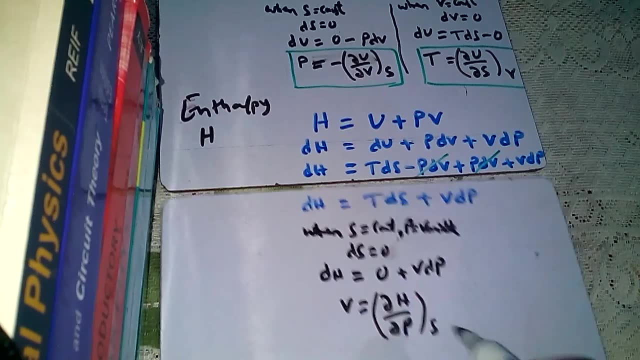 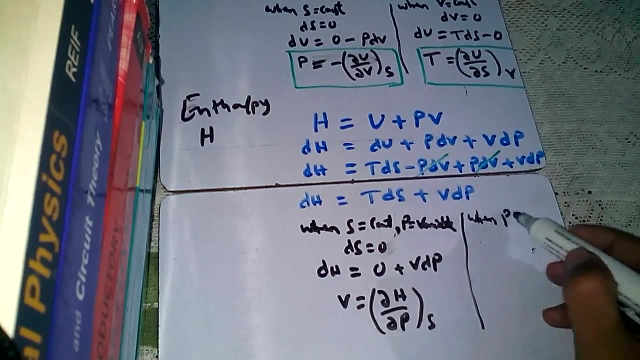 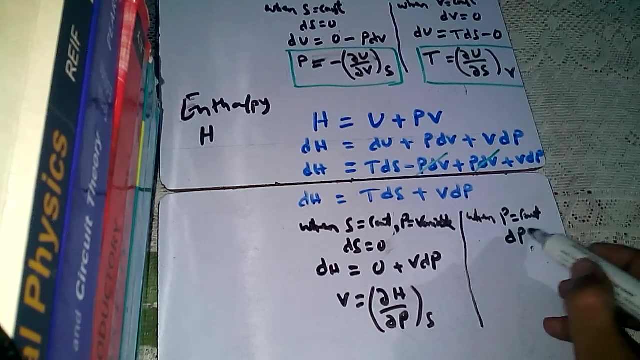 Okay, So V is equals to del H by del P under constant entropy. And we can have the second relation: when pressure is constant but entropy is variable, Entropy is not constant. Under this condition, dP is equals to 0.. And this relation becomes dH. 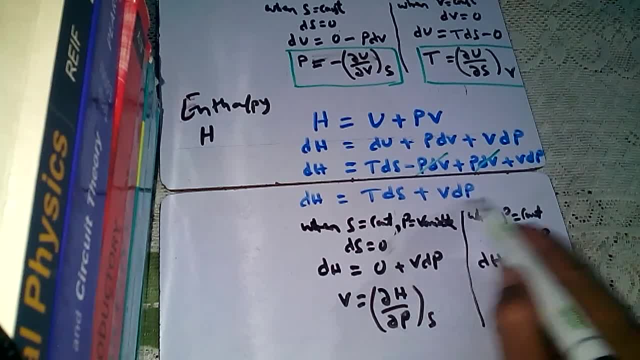 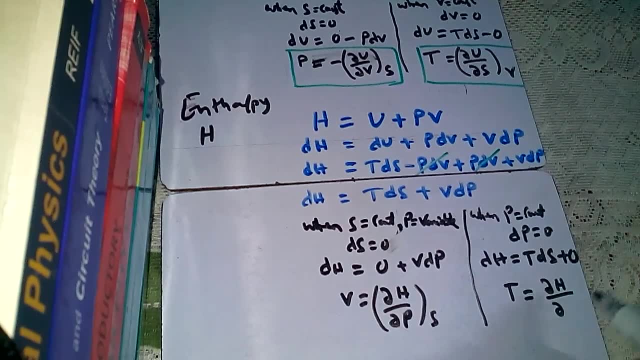 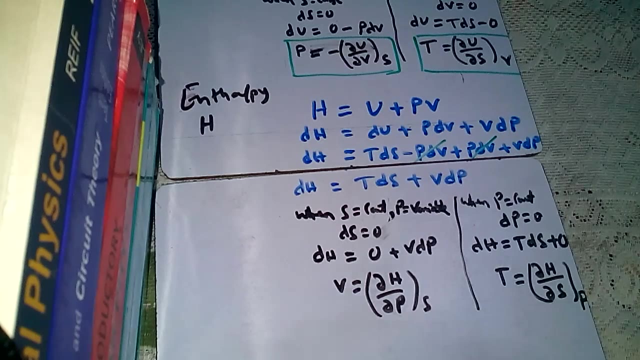 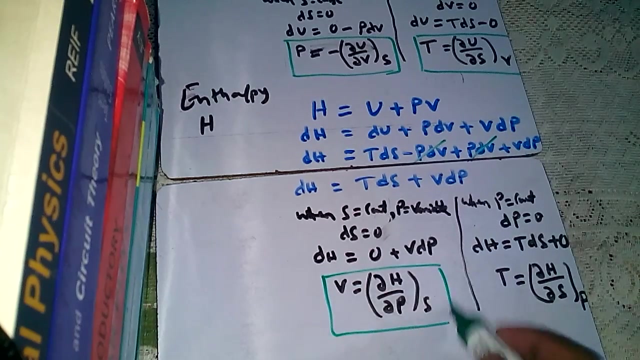 So this relation becomes dH equal to Tds plus. this part is 0 now And we can have: T is equals to del H by del S under constant pressure. So again we can have two relations, And one relation is for volume. 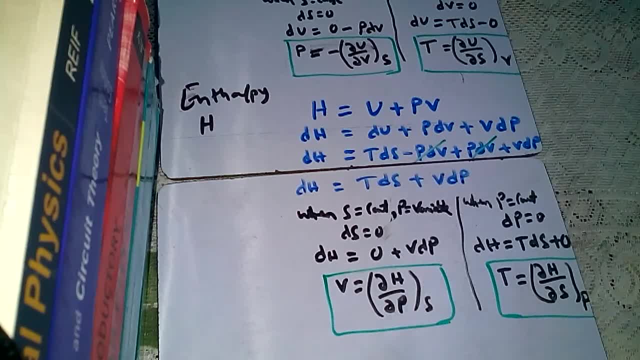 And the other relation is for temperature with enthalpy. So here it says that volume can be given as the rate of change of enthalpy, which is a potential energy, with respect to pressure under constant entropy, And it can also be given- the second relation- can be given by as the temperature, which is the rate of change of enthalpy with respect to entropy under constant pressure. 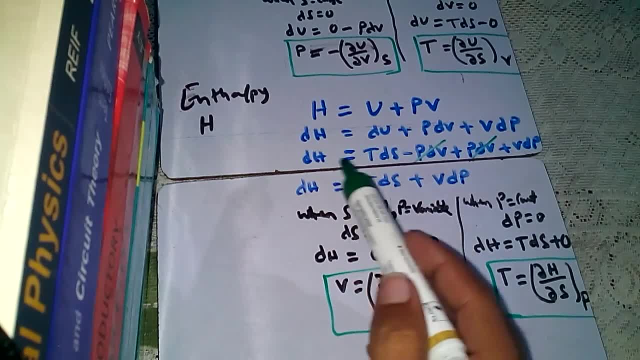 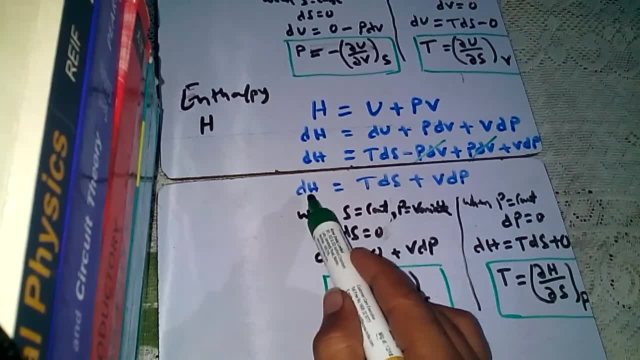 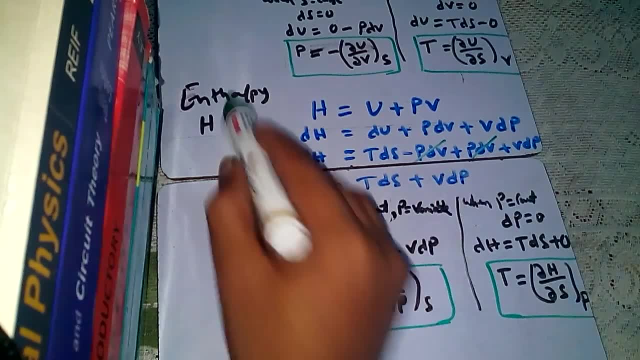 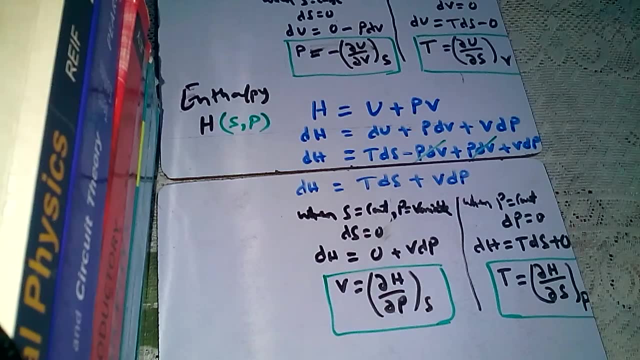 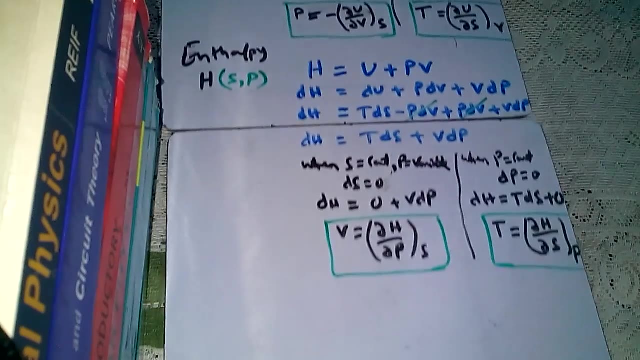 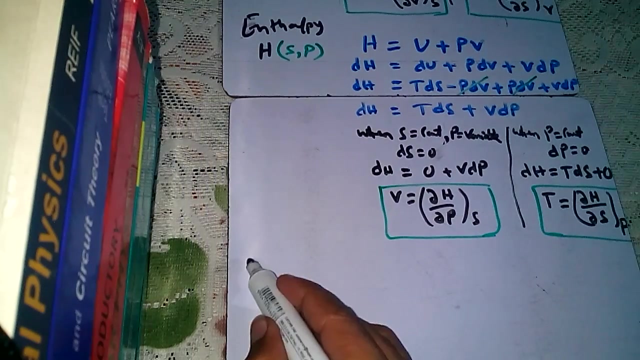 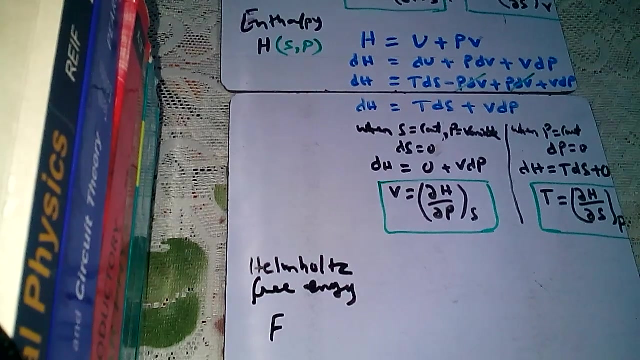 So this entropy and pressure, these are variable, And that's why enthalpy is a function of entropy and pressure. Now let us move to our next thermodynamic potential. so our next potential is him holds free energy and it is given by F and we. 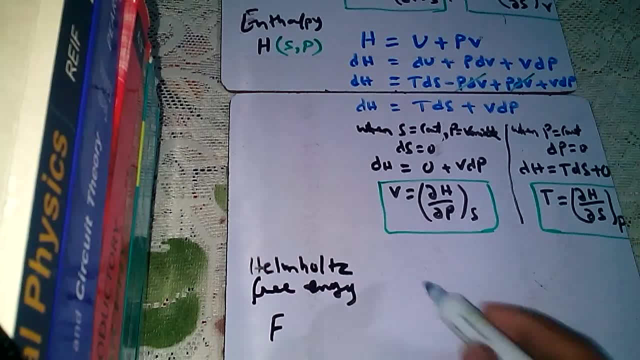 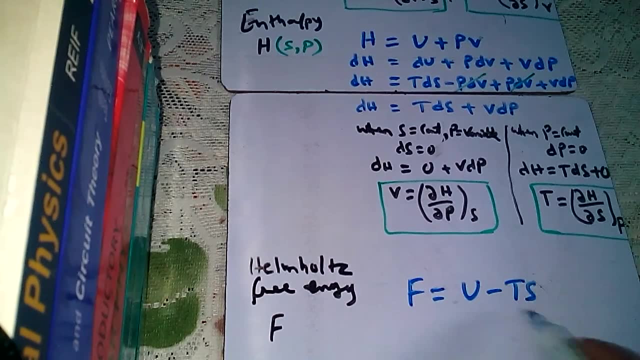 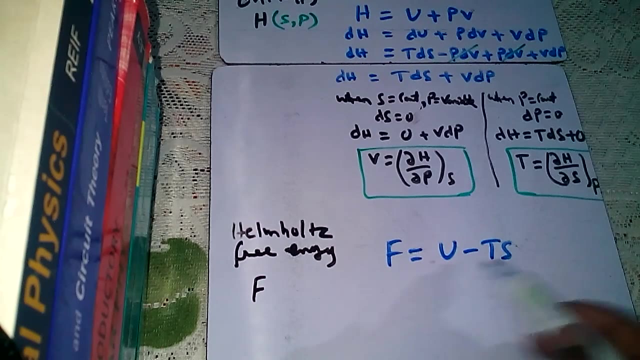 already know the relation for F. F is given by U minus TS. we already know this. now, one thing: F is equal to U minus TS. where from you can find it? you can find it from this. H is equal to U plus PV. always remember that this F, this, 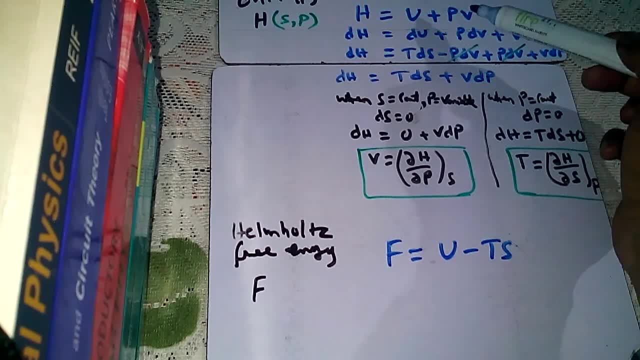 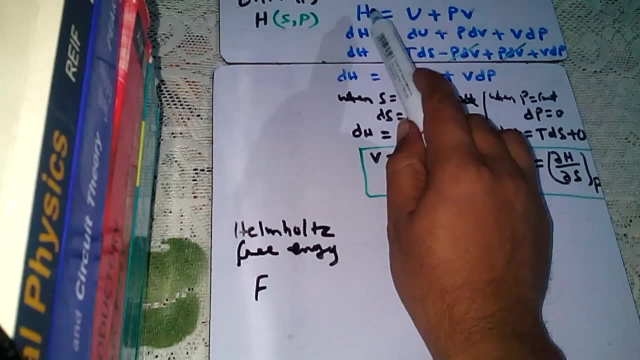 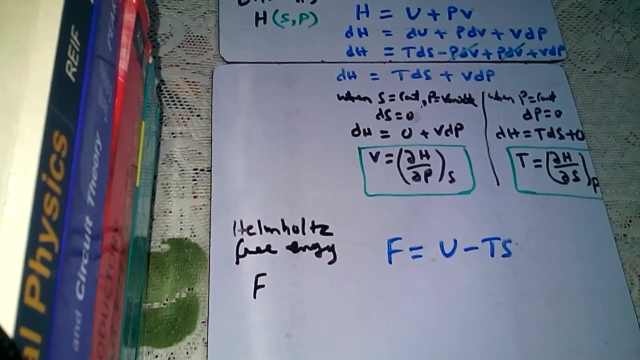 equation you can find from H equal to U plus PV by doing a transformation that is called the Legendre transformation. similarly, this enthalpy H equals to U plus PV. you can find this from the first law of thermodynamics by using the Legendre transformation. okay, but right. 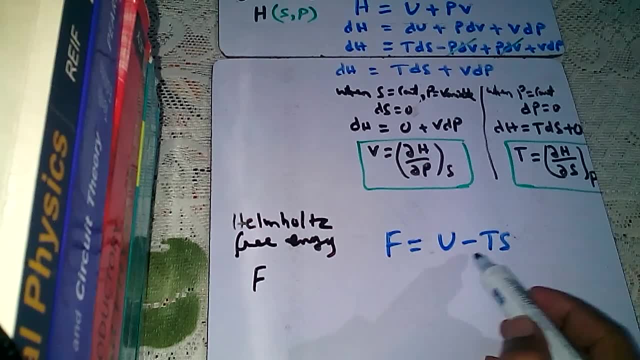 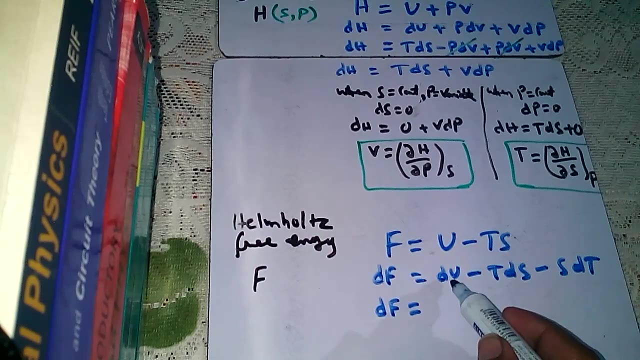 now we are not looking at that. now let's write: F is equal to U minus TS. now what we will do? we will differentiate on both the sides so it becomes: DF is equals to DU minus TDS, minus F, d, t. so DF is equals to D. you know, d you is. again we will use DU equal to TDS. 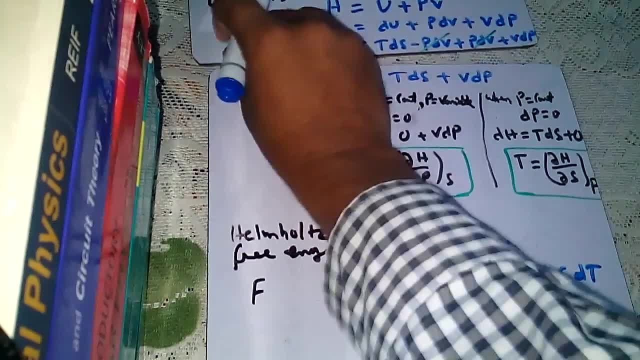 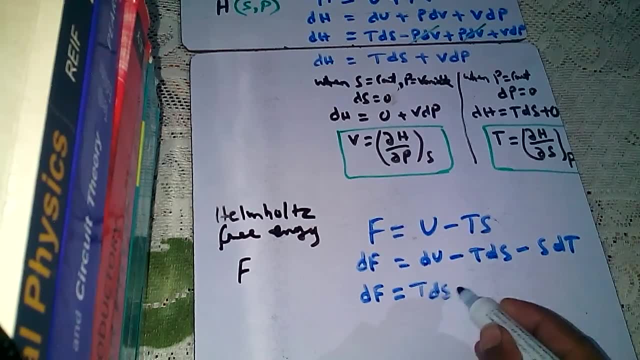 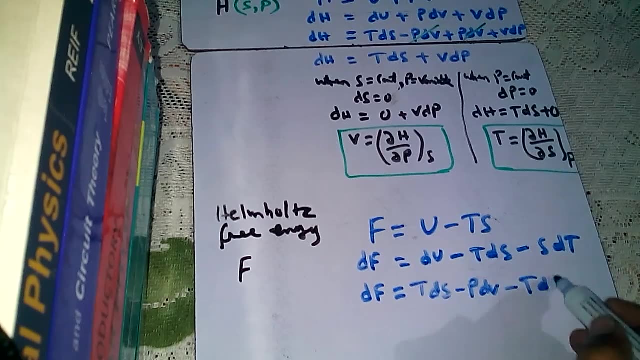 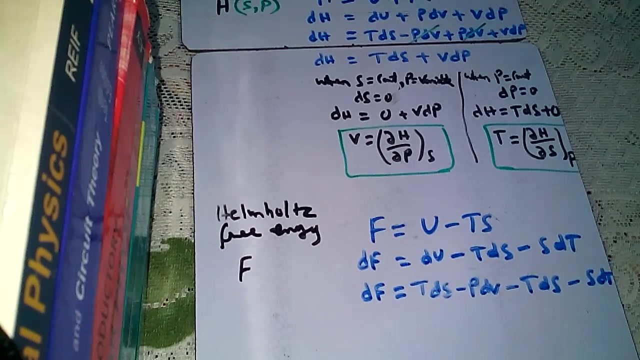 minus PD. been so. it is d DS minus PD. be. now we have mine. it's minus, tedious, tedious, minus, minus as dt. and you can see that this plus tds, this minus tds cancel- so we have df- is equals to minus pdv, minus s dt. again, we can have two relations from this. 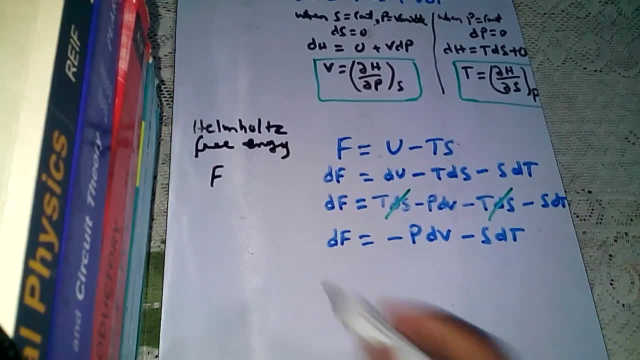 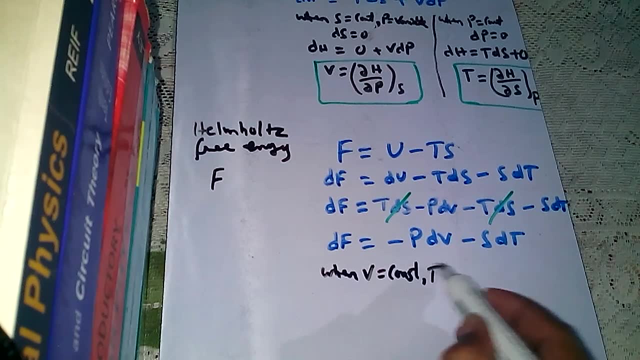 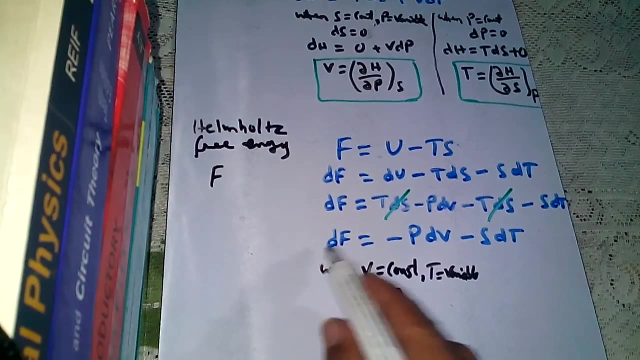 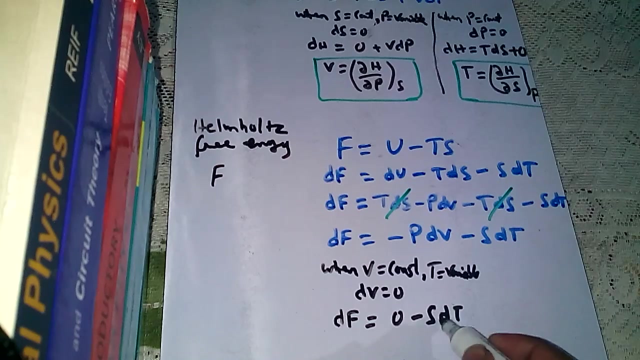 now the two relations under two conditions, when volume is constant and temperature is variable. in this condition dv is equals to 0 and this relation becomes: df is equals to this part is 0 minus s dt. so we have: s is equals to minus of 0 and dv is equal to minus pdv minus s dt. 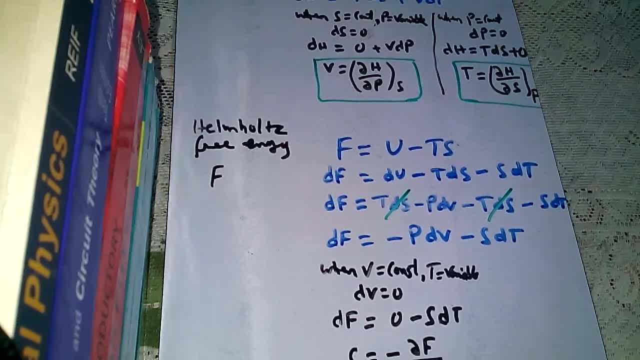 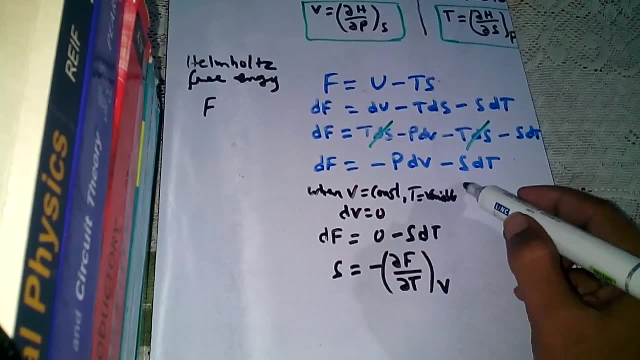 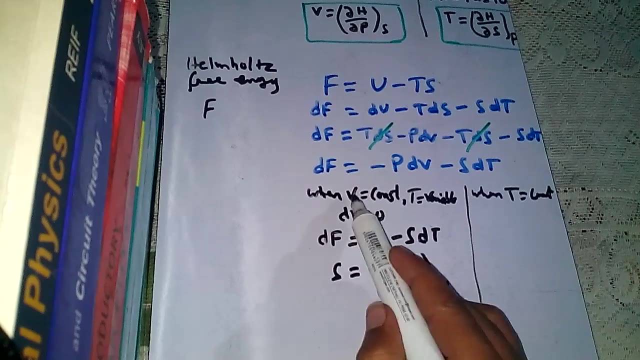 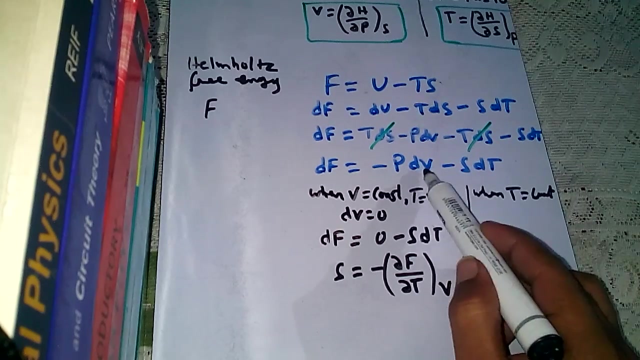 del f by del t under constant volume. and we can have the second relation by using the condition when temperature is constant and volume is variable. here volume is constant, temperature is variable. now we can take the condition of temperature to be constant but volume as variable, and in this condition dt. 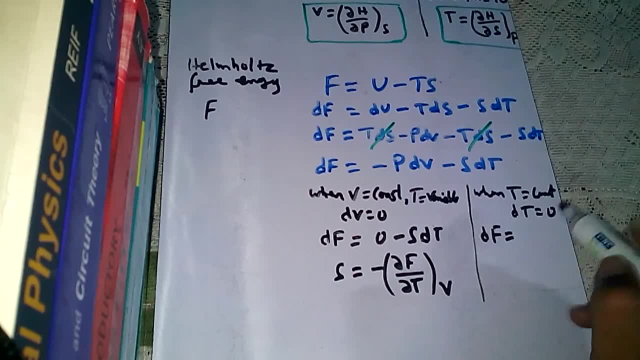 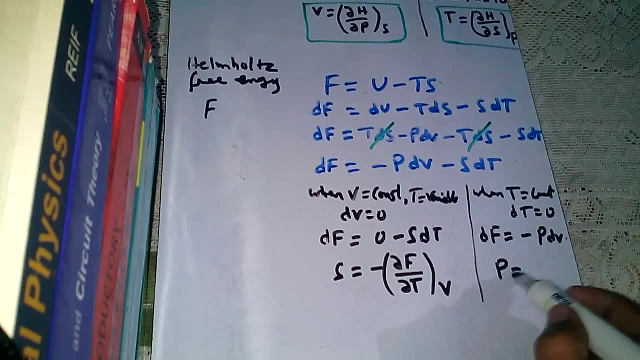 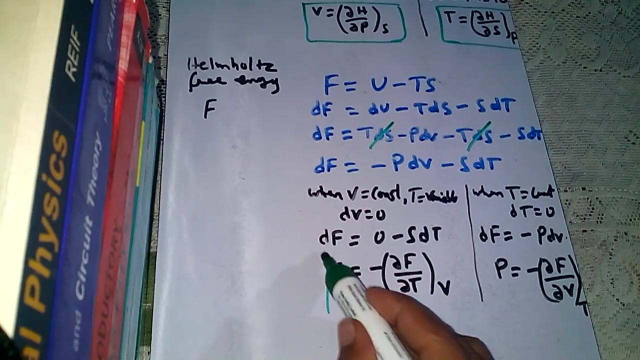 is equal to 0, then this relation becomes: df is equal to minus p dv, and this term is 0. okay, so we can have: p is equal to minus of del f by del v, and this is possible under constant temperature t. so again we have two relations. 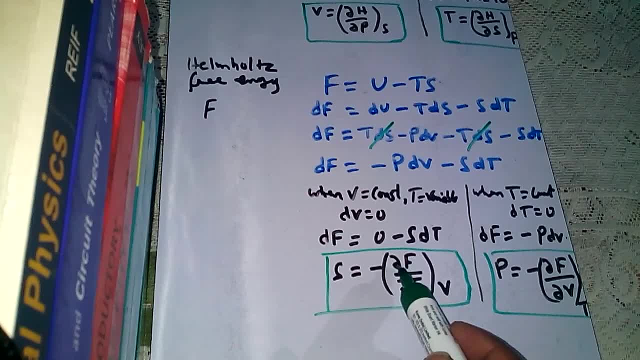 one relation says that entropy can be given as negative of the rate of change of Helmholtz free energy with respect to temperature under constant volume, and the second relation shows that pressure can be given as the negative of the rate of change of Helmholtz free energy. 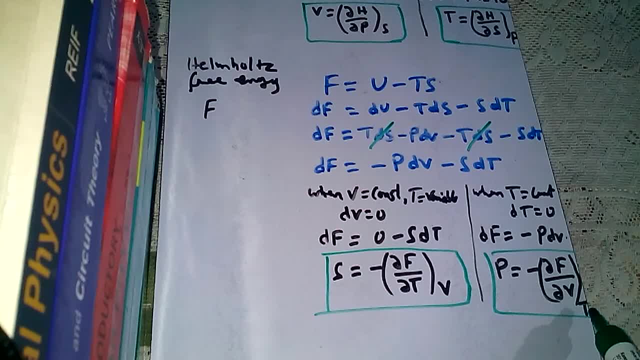 with respect to volume under constant temperature. so these are the two relations and they are very important. you should remember. now we have done thermodynamic potentials, we have seen. now the fourth one is Gibbs free energy. and one more thing, this: Helmholtz free energy. there is rate of change of Helmholtz free energy. 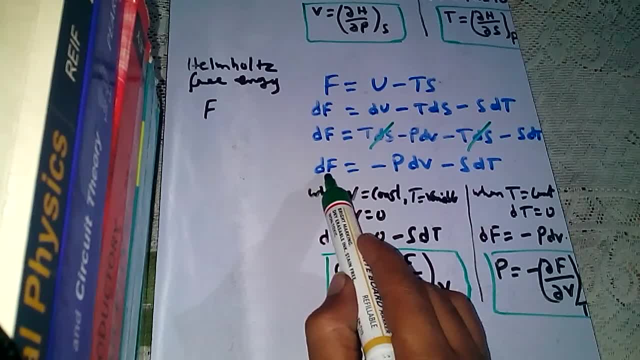 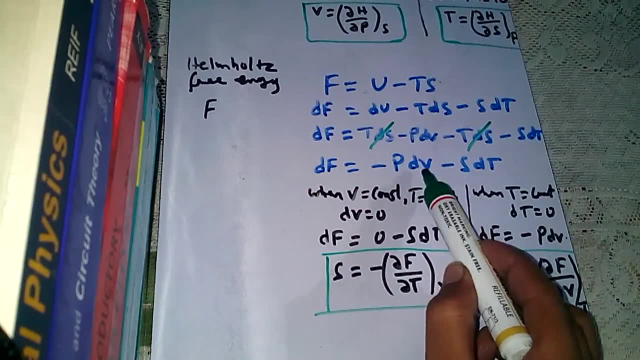 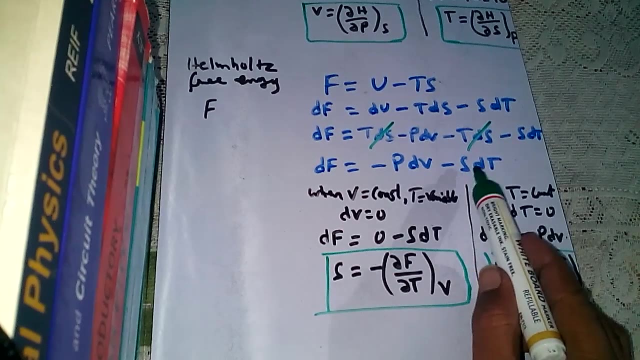 depends on the rate change of, not rate of change of, the change of Helmholtz. free energy depends on the change of volume and change of temperature. that means volume and temperature are now variable quantities, pressure and entropy are constants. drunk for this f and that's why this f. 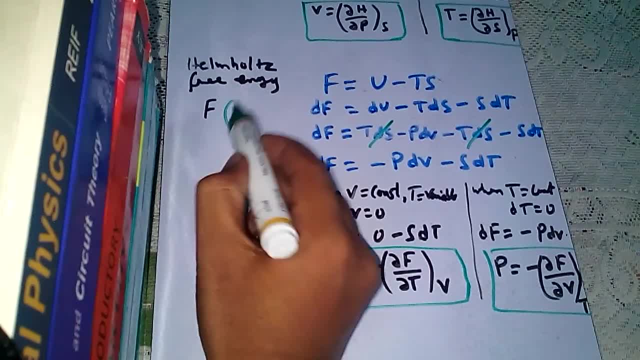 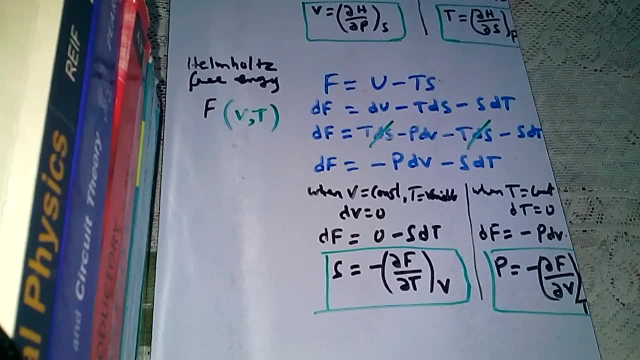 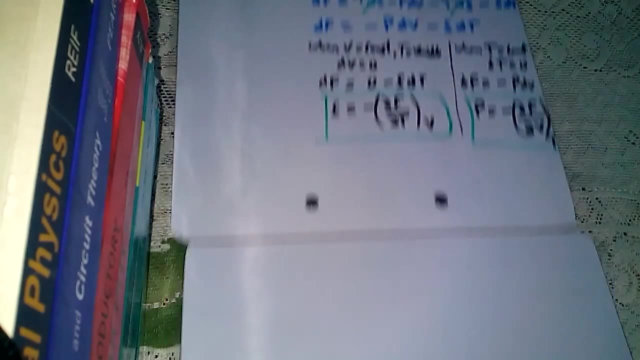 and that's why this f is generally the function of volume, and it is generally the function of volume and temperature. now let us move on this to our fourth potential: adian low pressure under constant tungsten rotation. now we have to come to this level of the temperature of free energy. 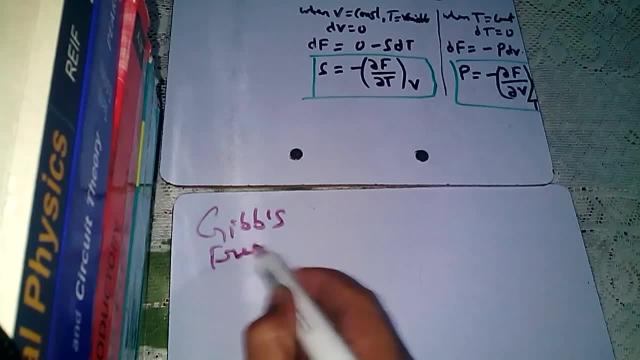 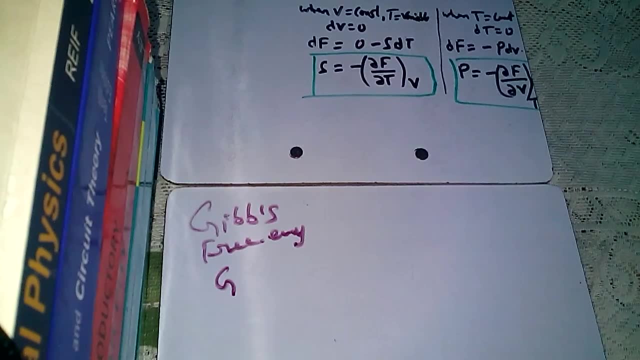 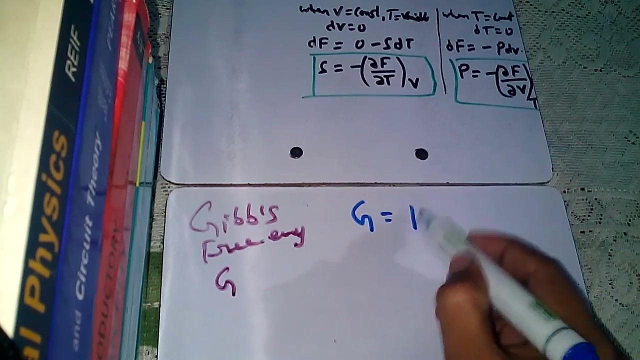 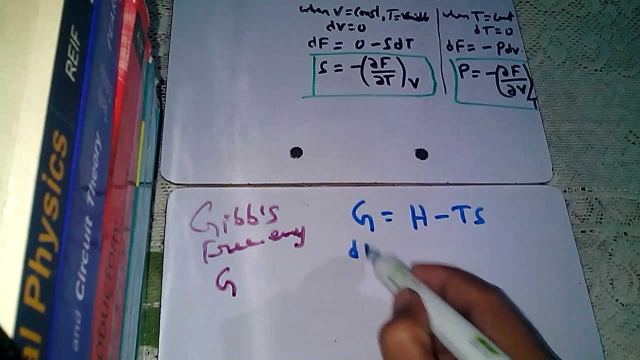 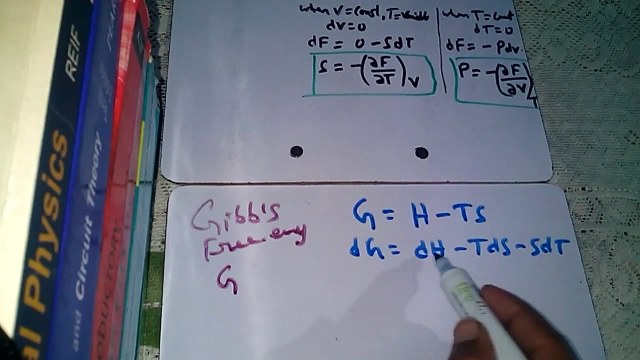 that is Gibbs free energy. it is given by G and we already know the relation for G. G is equals to H minus TS. we already know this. now what we need to do: we need to differentiate both the sides. so DG is equals to DH minus TDS, minus SGT. now what is DH? 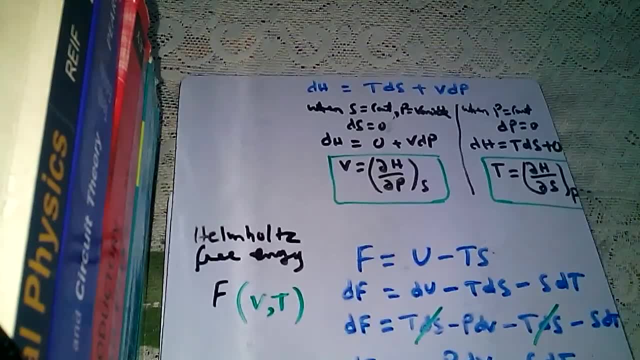 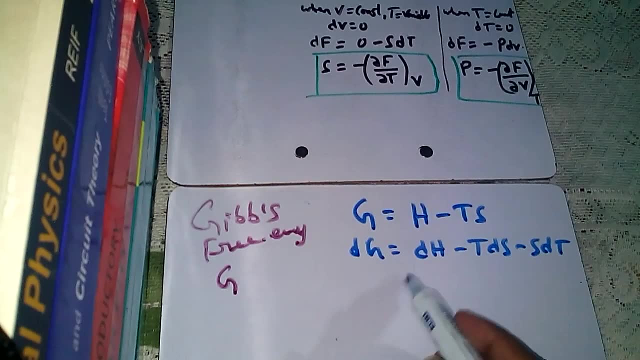 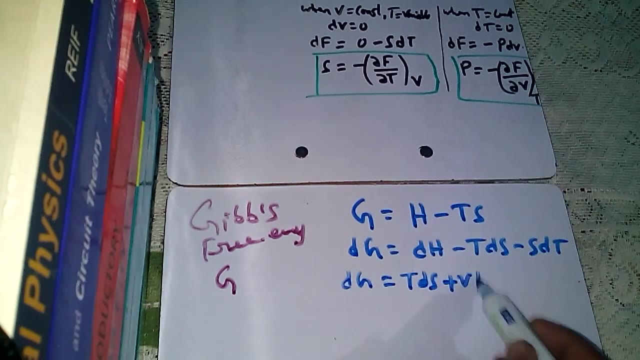 here we have seen that DH was TDS plus VDP, so we will use it. so we have DG is equals to. in place of DH, we will use TDS plus VDP, then minus TDS plus VDP, so we will use it. so we have DG is equals to. in place of DH, we will use 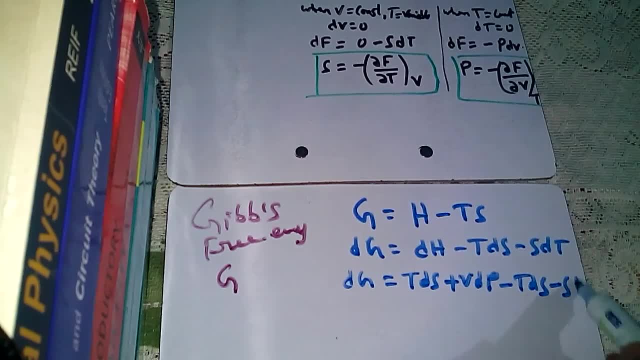 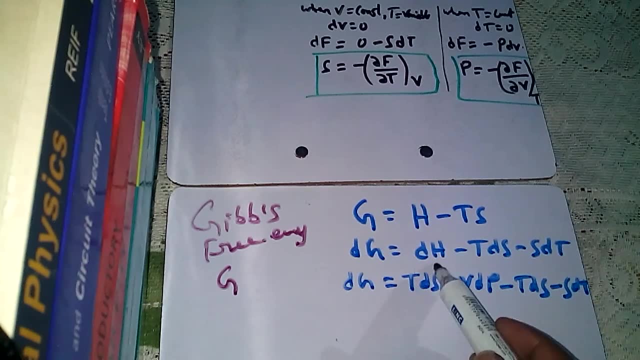 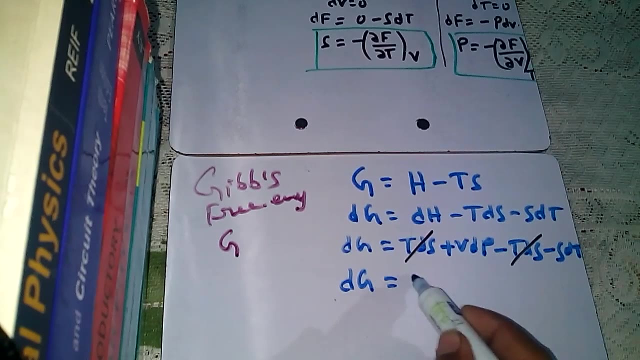 DS minus SGT and we can see that plus T DS minus TDS cancel, so we have D. G is. WE can see that plus T DS minus T DS cancel, so we have DG is equal to Emite gt. now again we can have two relations from two conditions now, when we also 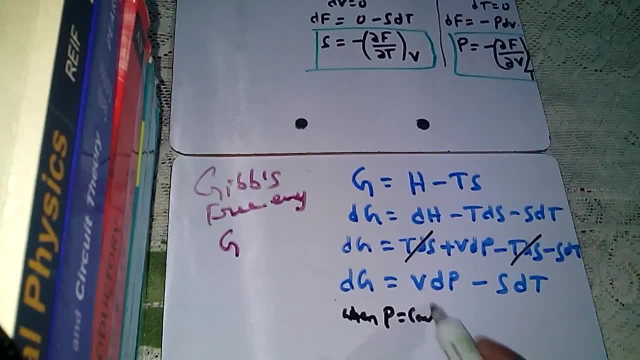 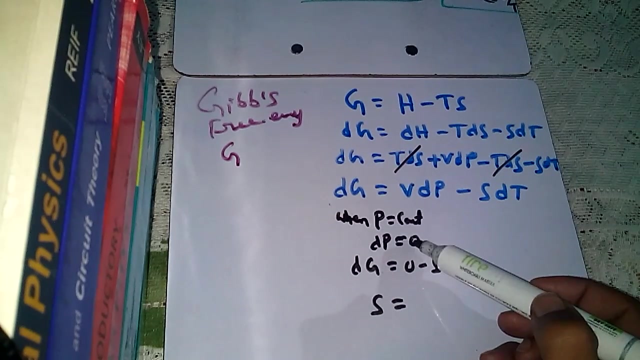 have relations very good. when we have zero relations. in case G is equal to TH, pressure is constant and temperature is variable, then dp is equal to zero and now the relation becomes: dg is equal to zero minus s, dt, so s is equal to: if p is constant, then dp is zero and this relation becomes dg is equal to. 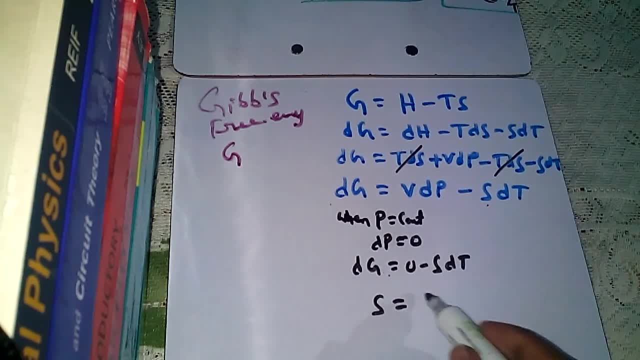 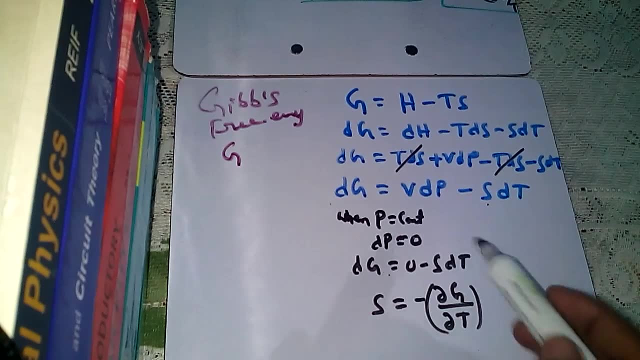 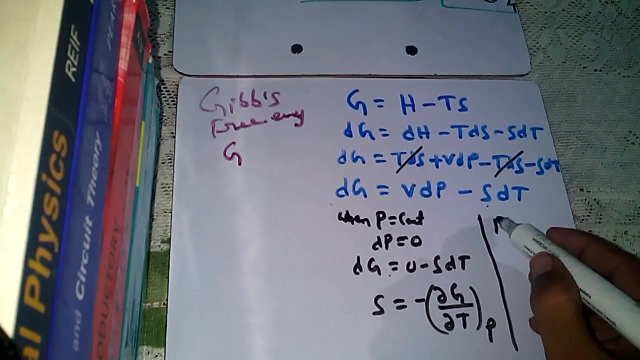 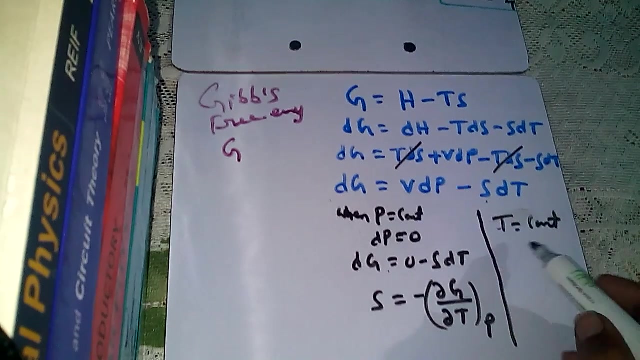 this part is zero minus s dt, and s is equal to minus of del g by del t. under constant pressure. and similarly, if we take temperature to be constant but pressure to be variable, then dt is equal to zero and under this condition the relation becomes: dp is equal to zero and s is equal to minus s dt and s is equal to minus of del g by del t.